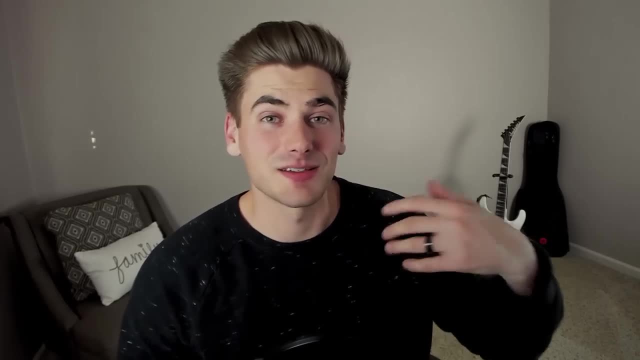 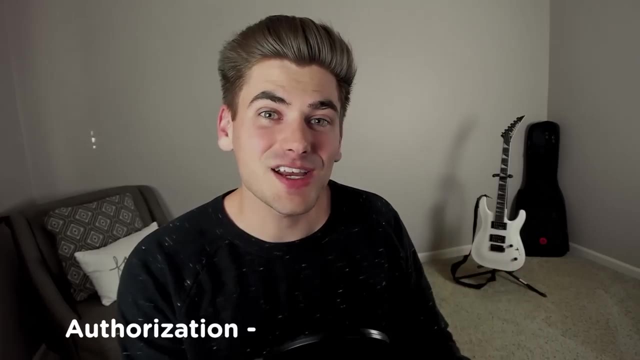 and now the web dev simplifies the web for you So you can start building your dream project sooner. The site knows that you are who you say you are, So if I sign in as myself, it knows that I am Kyle. and that's how you prove that you are Kyle to a website. This is step number one: Authorization. 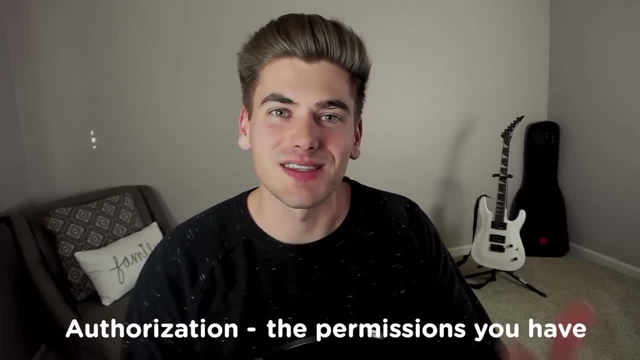 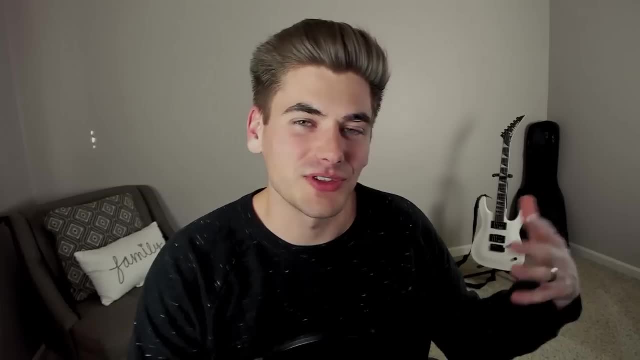 on the other hand, is just saying: do you have permission to do this thing? So there are different levels of users, different roles and permissions. For example, you could be an admin user, you could be a guest, you could be just a normal default user, and these permissions are tied to who you 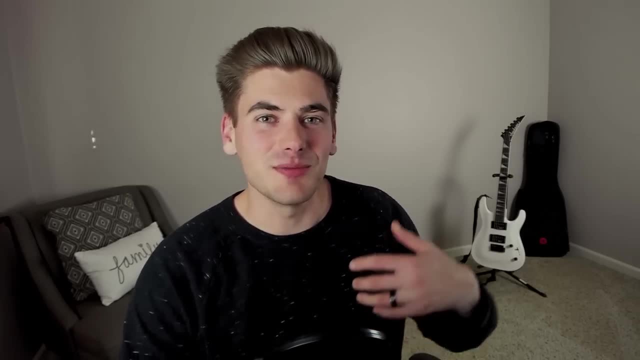 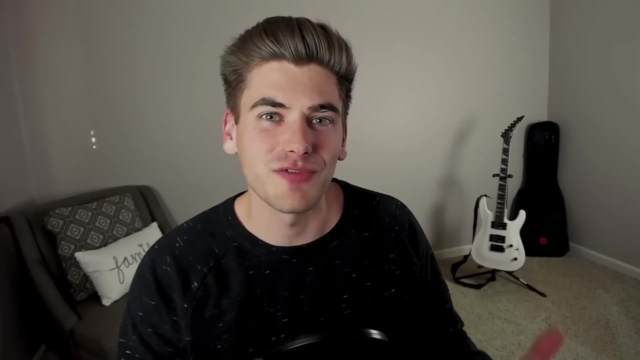 actually are. So me, as Kyle owning my YouTube channel, I am the owner of this channel, While when you are on YouTube and you view my channel, you can only view it as a viewer. like you can't edit or delete any of my videos, So the ability for me to edit and delete videos is tied to 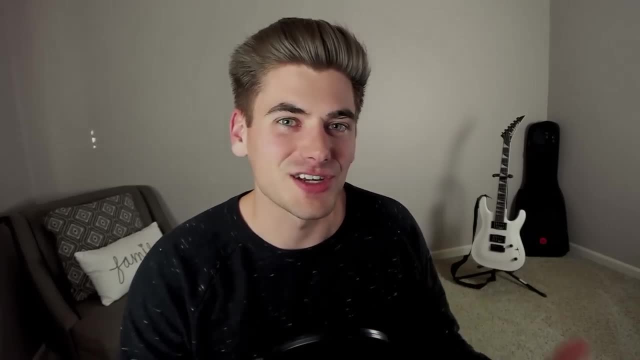 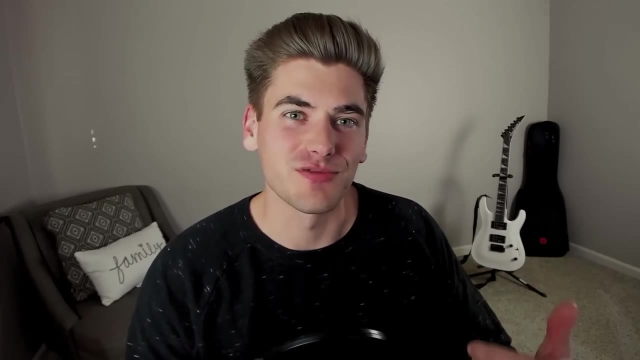 permissions that I need to be authorized to do, which is where authorization comes from, And this is essentially step number two. Once you are authenticated as yourself, then the server can authorize you to do different things. So that's the difference between authentication and 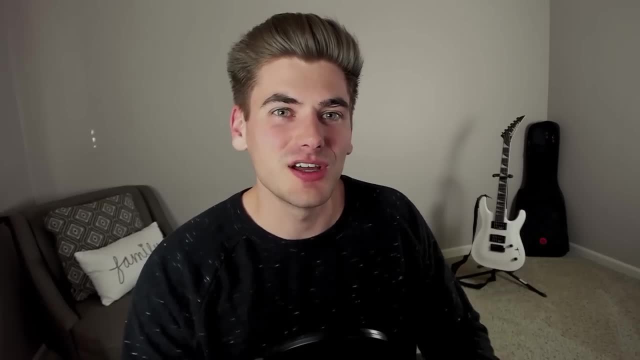 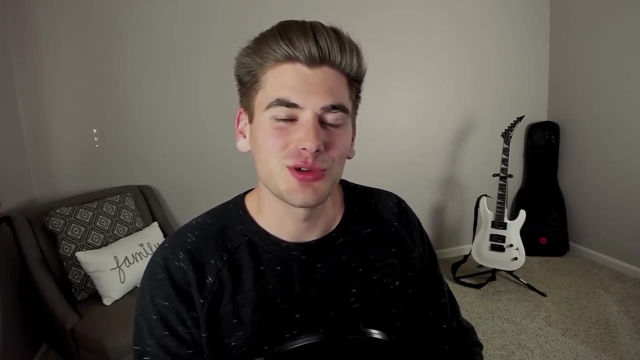 authorization. It's okay if you're not 100% clear on the terminology. just understand that there are two different concepts: One is logging in and one is having permissions. So now that we understand the difference between these two terminologies we need to understand. 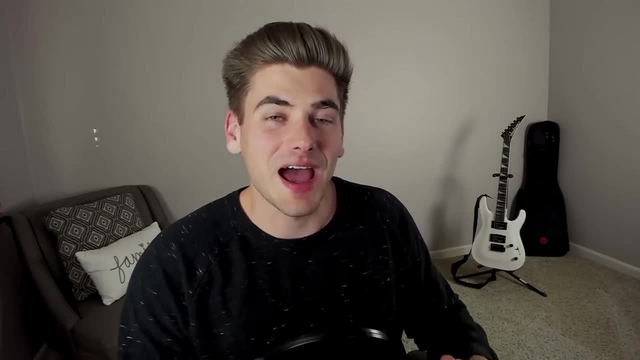 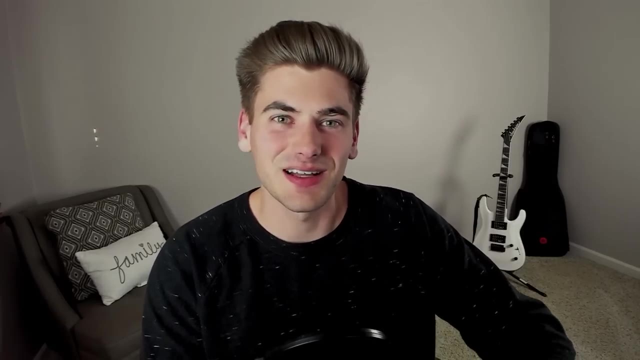 exactly how auth works And the whole idea behind auth is that it happens on the server. A lot of people think about auth on the client like, okay, you know, I have this user, what can they do, What buttons can they click? but everything to do with auth happens on the server, And the reason for 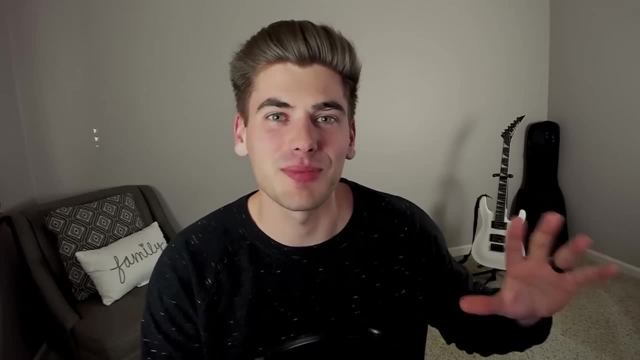 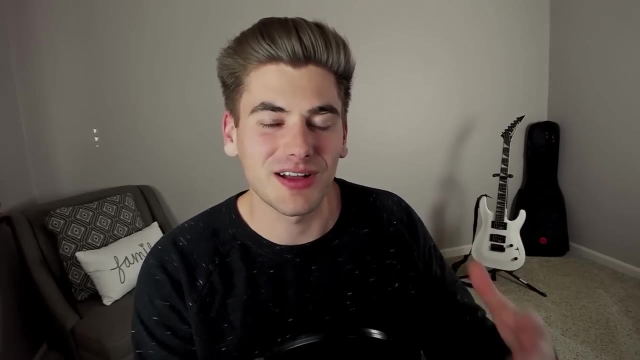 that is, you cannot trust the client. So everything with auth has to happen on the server, And the two different processes, authentication and authorization, have a little bit of a workflow. So the way the client can communicate with each other is by request. So if you want to log in, the client is going to. 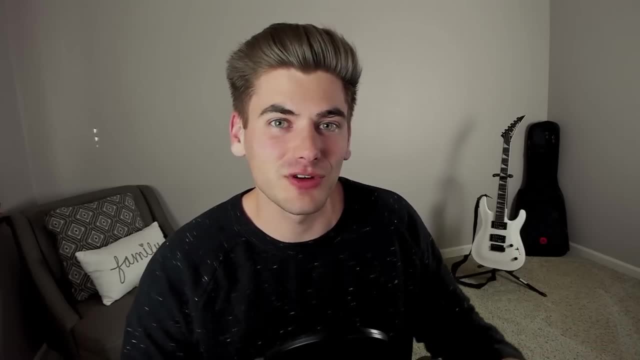 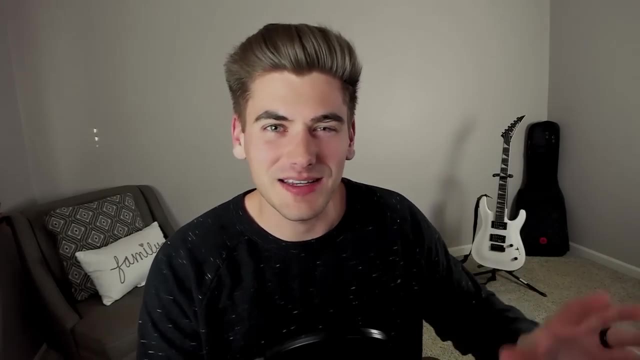 send a request to the server with your email and password and ask the server: is this person you know able to log in And who is this person with this credentials? then the server will say: you know, this is who they are. So it's going to be that type of process And to talk about specifically. 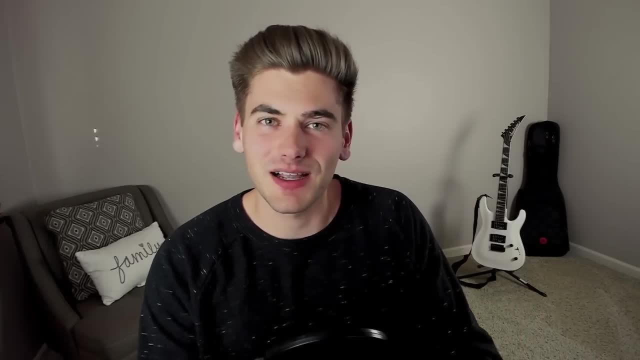 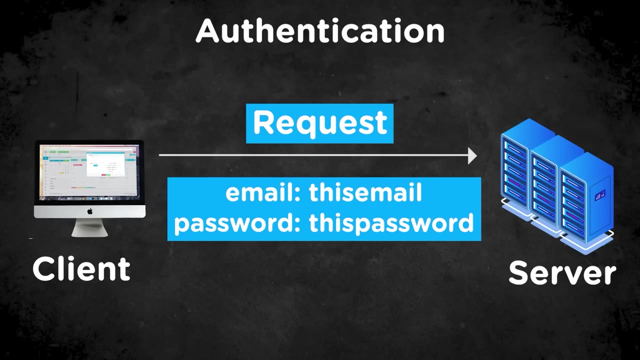 authentication. that's going to be the login process, And what happens, like I already mentioned, first step is the client sends a request to the server that says: I have this email, I have this password. is this person a valid user? And if so, 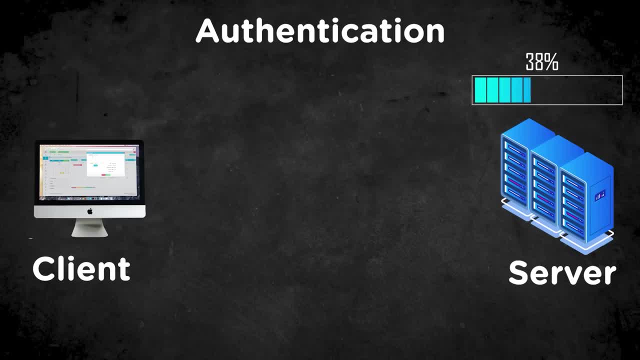 are they? Then what happens on the server is it's going to crunch that information and determine: does this user exist? If this user does exist, well, it's going to send that information back down to the client. it's going to say: hey, this is John. And what happens also on the server? 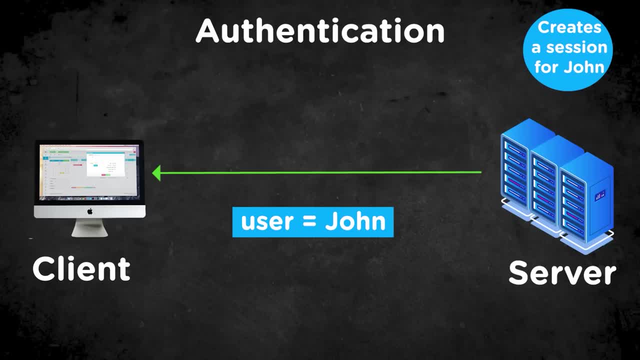 if this is correct, is it's going to create a session? The session is just a unique ID specifically associated with John, And this unique ID is how the server determines that this is always you when you make further requests. So it's going to send down that specific ID saying: 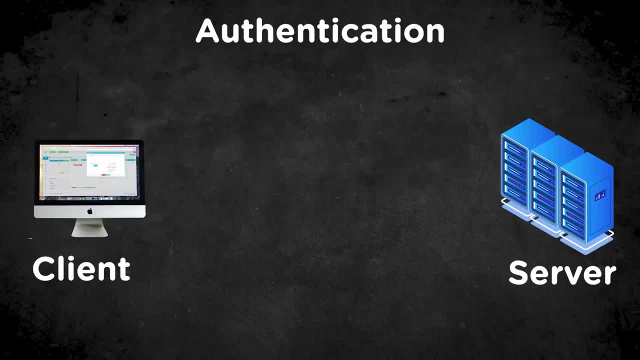 that this is John and it's going to be like: yep, you're good to go On the client. you're then going to take that special ID and it's going to be saved, most likely in a cookie. That way, every time you make a future request that requires authorization. 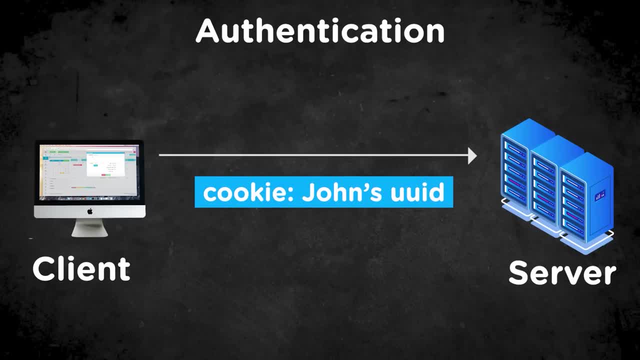 that cookie that has your specific ID for John is going to be sent along with your request. That way, the server knows that this is coming from John. Now, in the other scenario, where, for example, the user does not exist, the server is just going to say: hey, email password. these are incorrect. 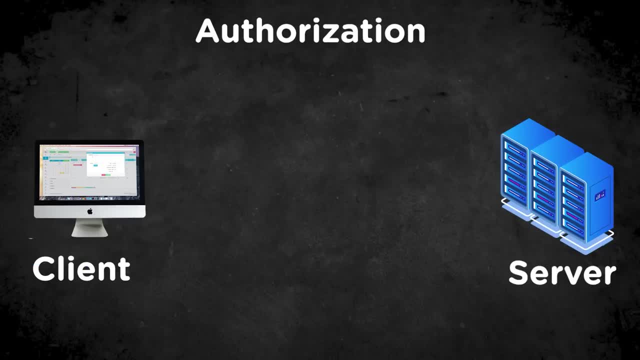 you know, try to reenter it. super basic stuff like that. Now for authorization. we touched on this just a little bit in the previous section. but what happens is the client is again going to make a request to the server. Let's say that you click on a button that's going to allow. 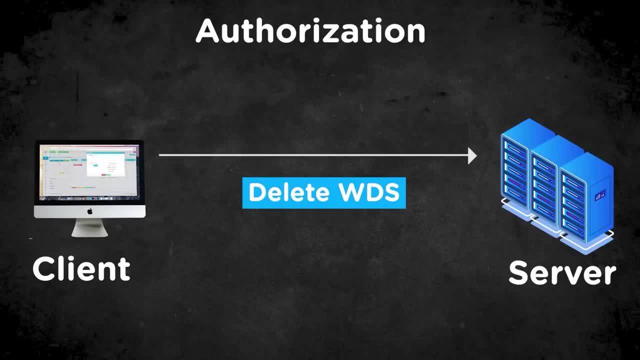 you to delete my YouTube channel. Well, I have permission to do that, but nobody else does. So it's going to send up that little cookie that we talked about earlier, that ID that says I am John. It's going to send that up to the server and it says: does John have permission to delete? 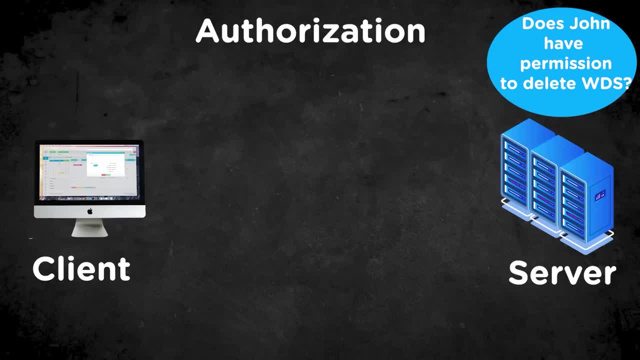 Web Dev Simplified's YouTube channel. Obviously- or at least hopefully, John does not have permission to do that, So it's going to send down an error. that's like John does not have the ability to do this. Or, for example, if you're trying to query a list of information and you send along your ID. 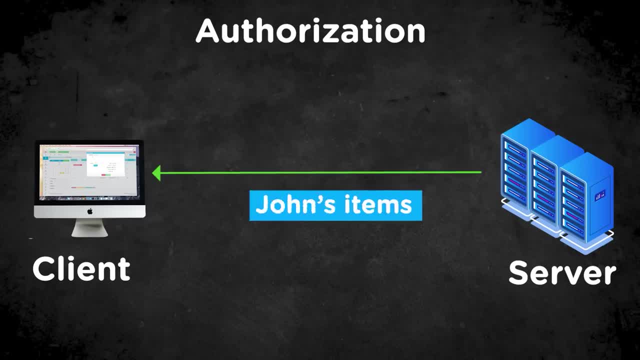 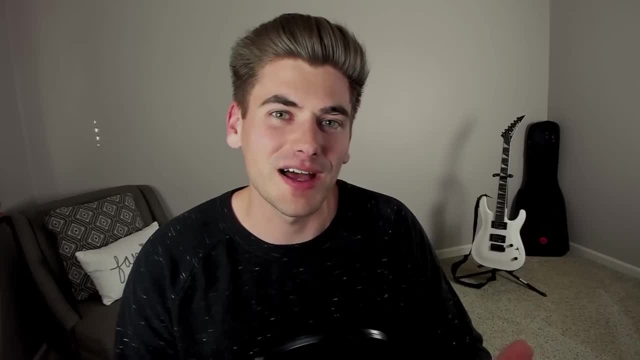 that is saying you are John, it's only going to return to you the items that you are allowed to access from that list of information. So if you're like a teacher of a classroom, it's only going to return to you the students that are in your classroom instead of all the students in the. 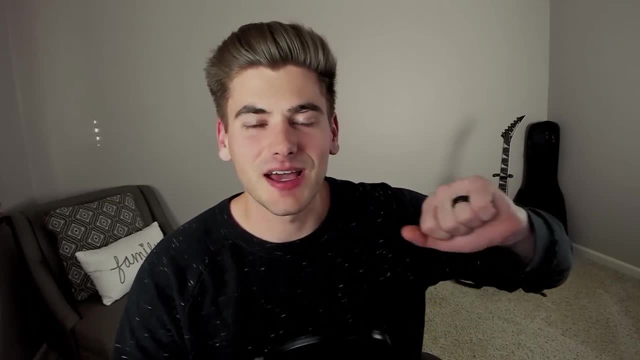 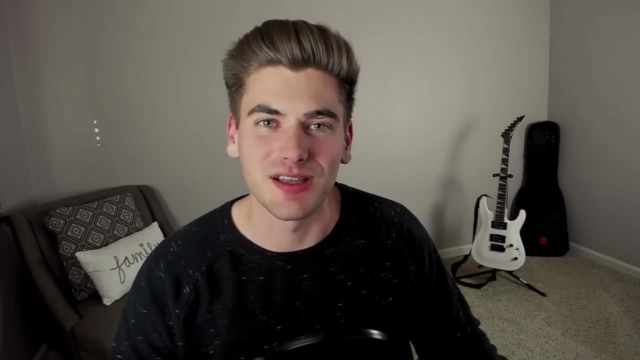 entire school. Now, obviously, if you pass up this ID and this ID for John does not have access to do something, it's going to give them an error. Otherwise it's going to, you know, return that data or allow them to do that specific thing. Now, the important thing to realize about these: 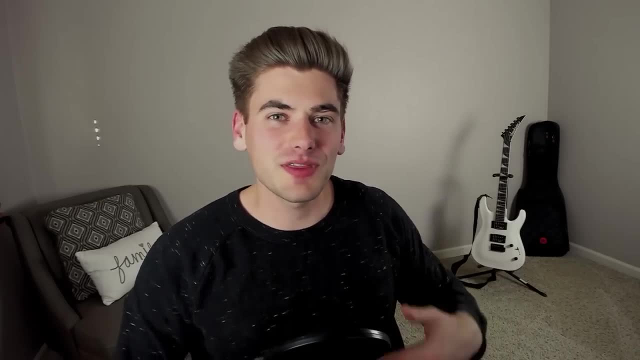 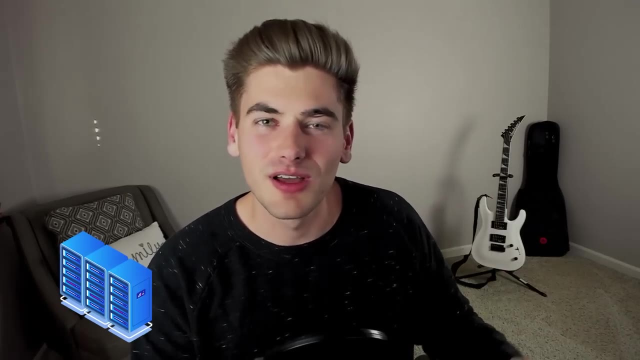 two different examples of authentication and authorization. is that everything that is validating that the user can do what they want to do, or validating the users who they say they are- is happening on the server? We're not checking emails and passwords on the client and we're 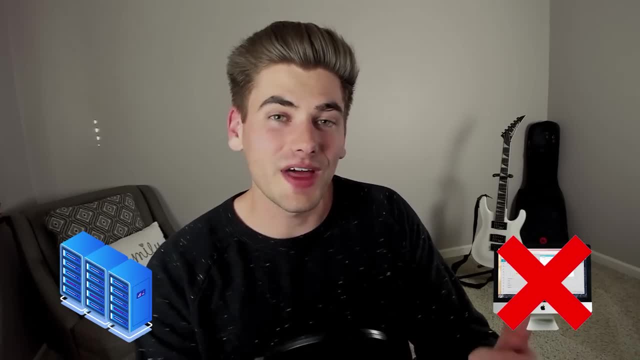 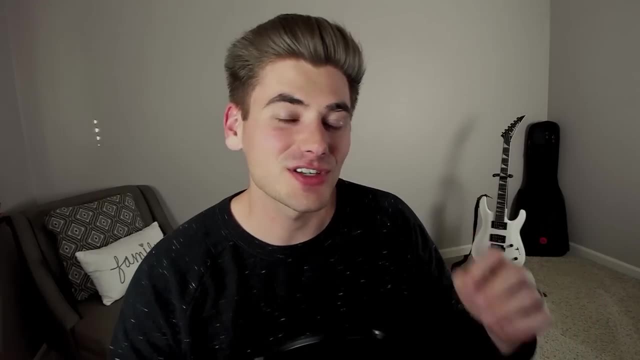 not allowing people to delete my YouTube channel from the client. All of that happens on the server And that's the key. Whenever you do authentication, all the validation, all the source of truth has to come from the server, since you cannot trust the client Now, it is 100% okay to use like. 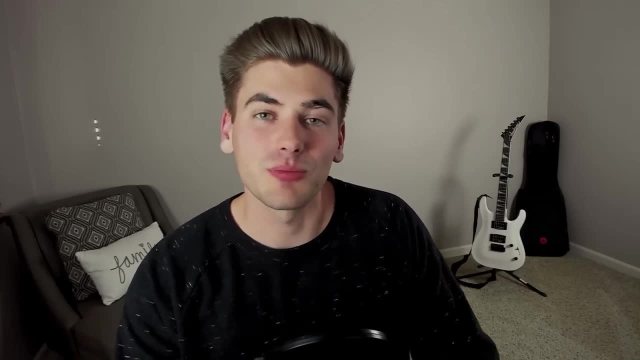 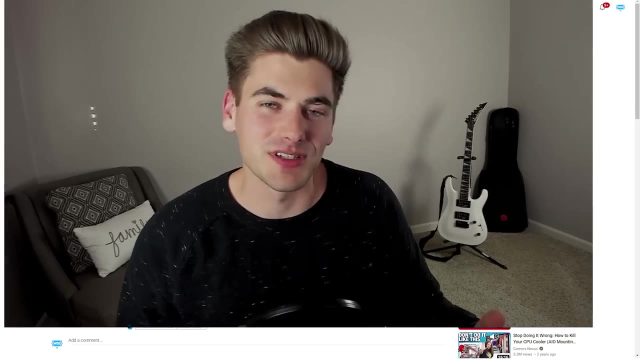 Boolean variables like isAdmin, to be able to show and hide different parts of your UI. For example, you may be able to want to show a delete or an edit button where a normal user doesn't have that. For example, when I go on YouTube it shows an edit video button which has a link for me to 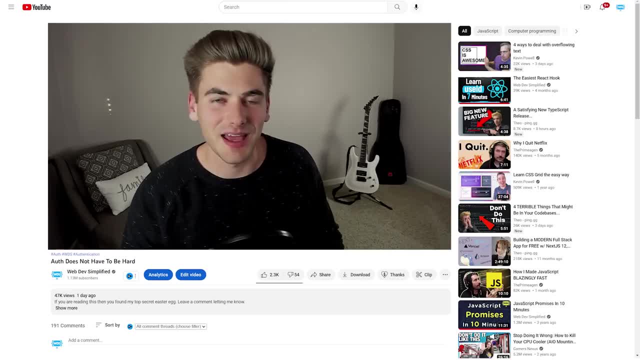 edit any of my videos underneath my video And if I click on that link it allows me to edit the video. But you know that could be behind a flag that says like: is this Kyle Cook? If it's not Kyle Cook, then don't show this. And if you change the UI, you change the client side, so that that. 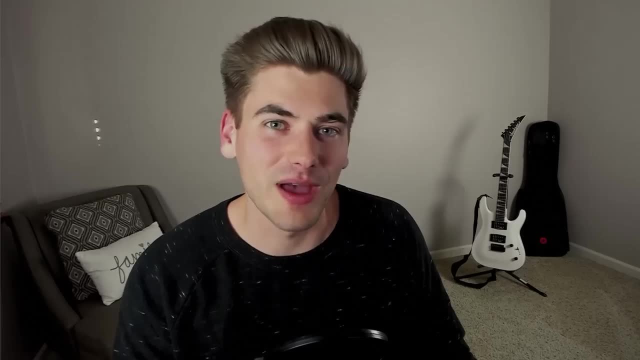 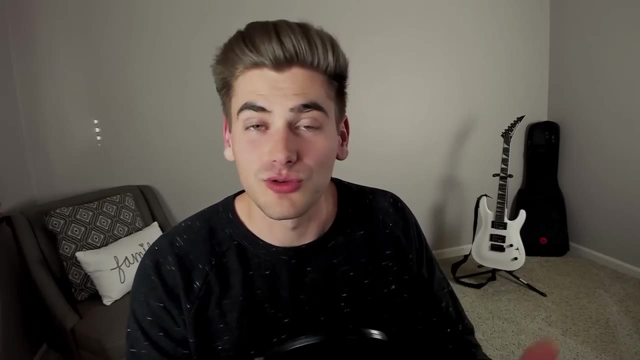 button shows up for you and you click it. obviously, YouTube's not going to let you edit my video. Instead, it's going to throw you an error. So it's perfectly okay to show and hide things on actual, you know, user's data or the user information, But because you can change that, 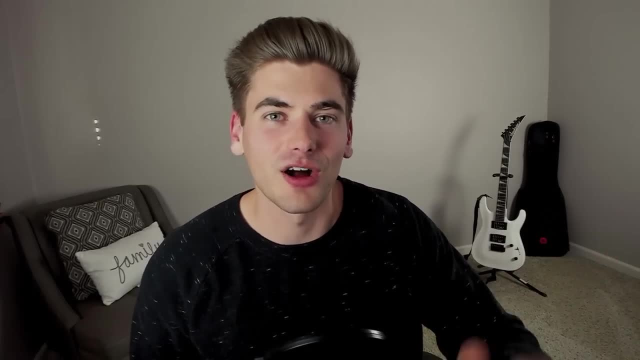 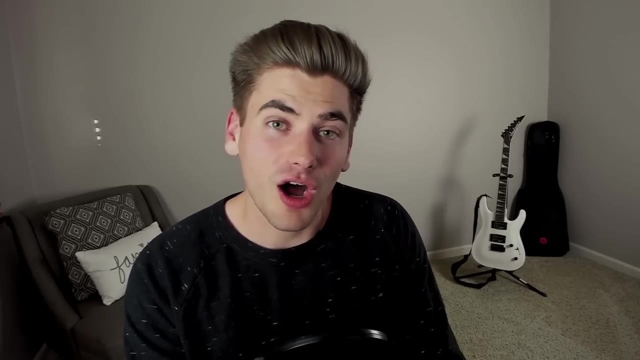 information. I can go in and I can, you know, change my flag to admin flag on the client. You don't want to actually trust any of that information, So you can show and hide things all you want, But the actual verification and authorization of if the user has access to that. 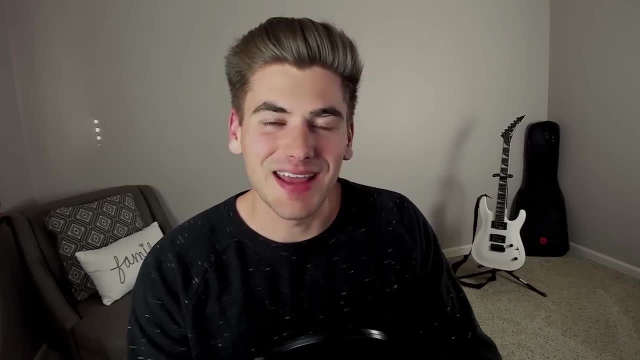 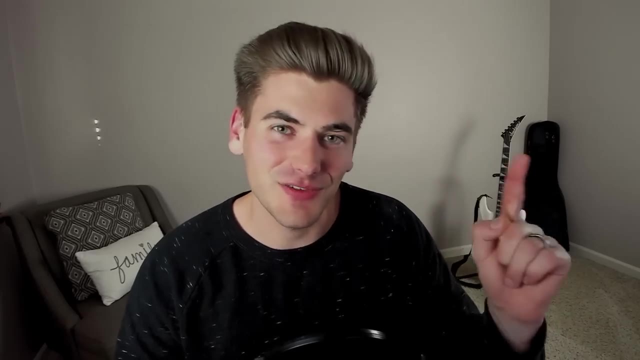 information needs to be handled on the server. So if you go ahead and add an edit video button underneath of my video by changing around your client side code and you click on it, the server of YouTube is going to tell you: hey, that's funny, You tried to do that, but we're checking you on the 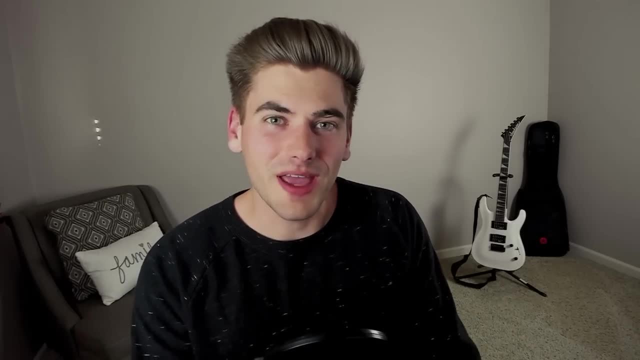 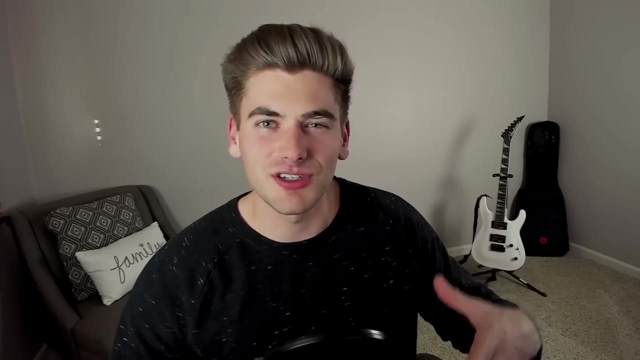 and you cannot do that at all. So just kind of to reiterate that point: it's okay to use the actual user information to hide and show and do different things based on your UI on the client, But the actual verifications and checks all need to happen on the server to make sure they can do the things. 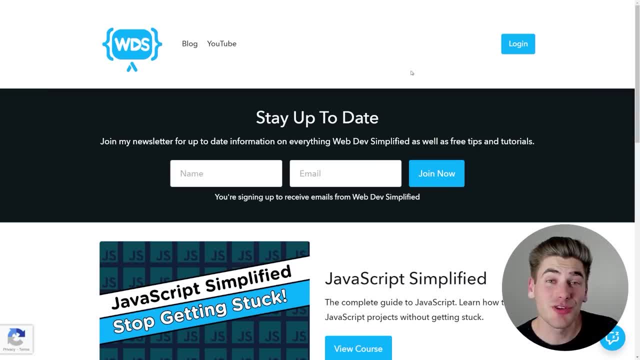 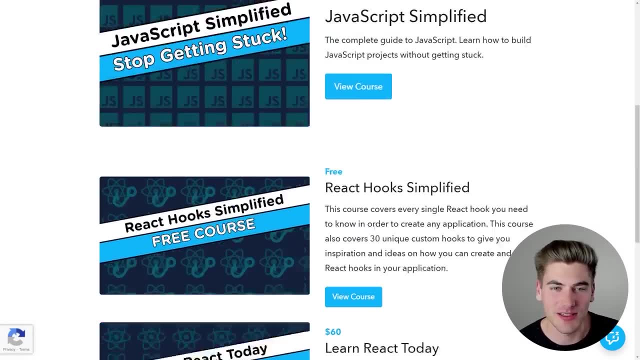 that the client says they should be able to do So. now that we understand how all these different processes work, I actually want to show you working on a live website. So we're actually on my own website for where I sell all of my different courses And we're just going to log. 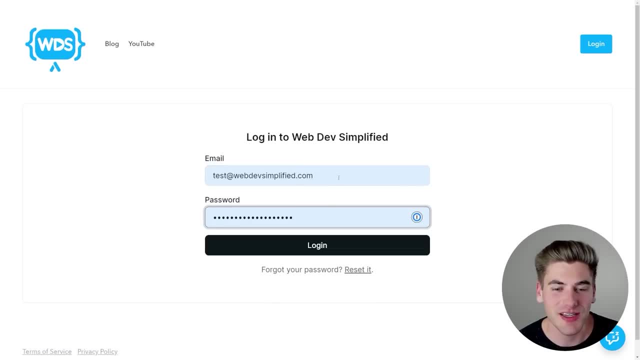 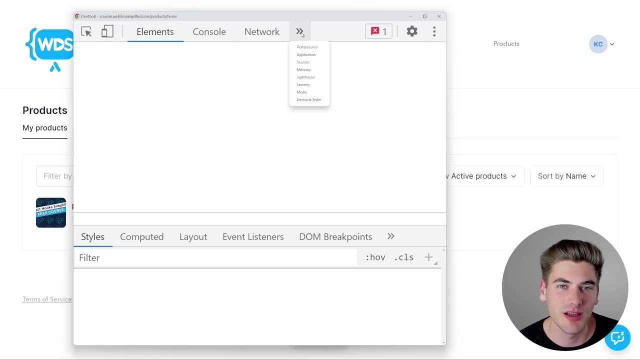 into an account. So I have an account on this website. It's just a test user I use for testing things. I'm going to click log in here and you can see that I'm logged in and I have access to this one free course. Now, if I inspect the page real quick, I go over to the application tab. This is: 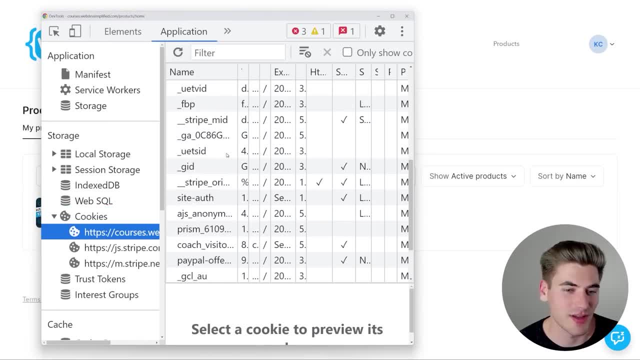 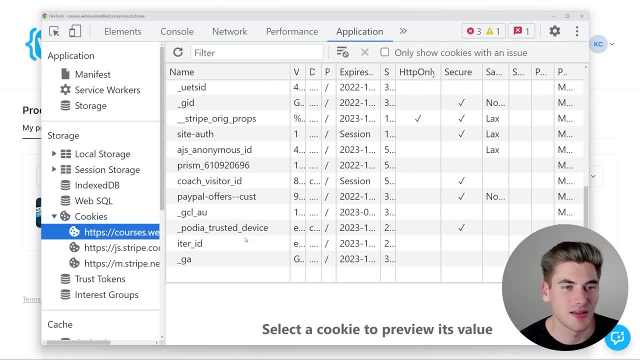 where you can see all the information, And if we go onto the cookie section, for my course, obviously there's tons of stuff, But the thing that you're going to see- if we just expand this a little bit, that's really important- is we're going to have to find, essentially, our ID, And I already know for 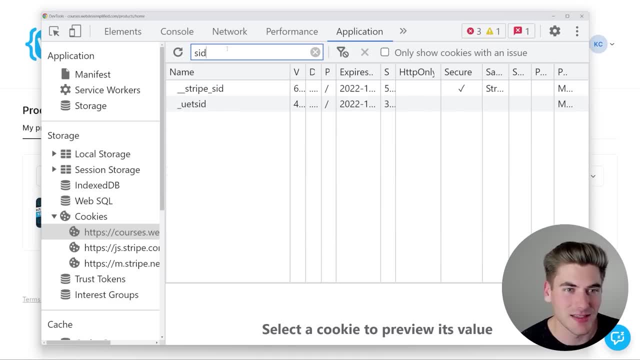 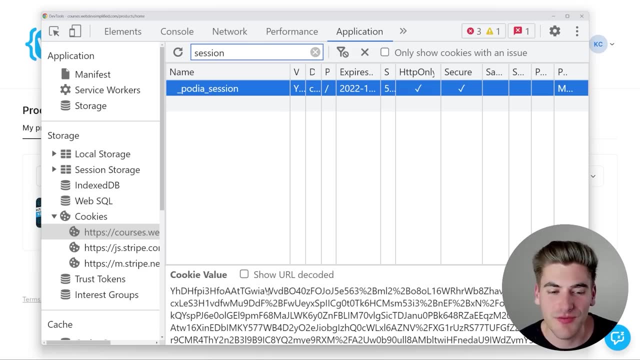 a fact that this is usually called something like session or SID, And in our case if we just say here session, you can see we have this underscore Podia session. If we just click on that, you can see we get this really long cookie value And this is just a bunch of jumbled up text. It really 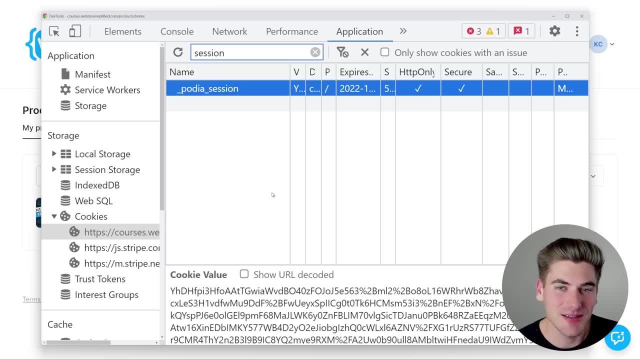 doesn't matter what this is. It's just a unique identifier that's saying: this is me And the important thing is, if I delete this, it essentially is like the same as logging me out, because this is what the server- or, I'm sorry, the client- sends up to the server every time I make a request. 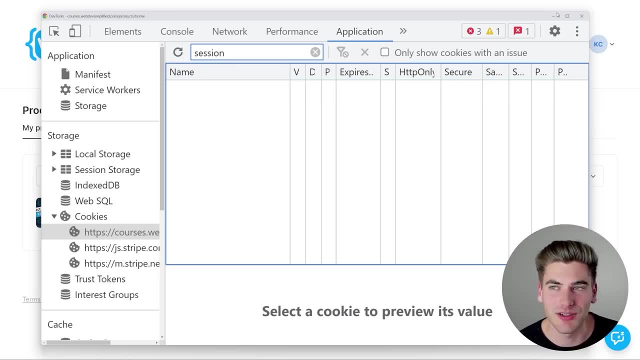 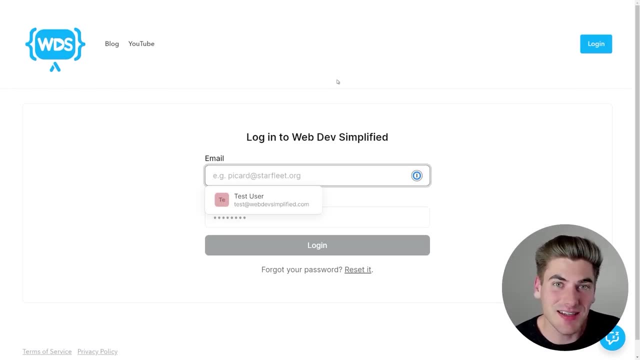 to verify that this is me. So if I delete this and I just come over and I refresh my page by hitting F5, you're going to see immediately it's logged me out. And that's because that session ID that is being stored in my cookies is what is actually verifying that I'm logged in and verifying who I'm. 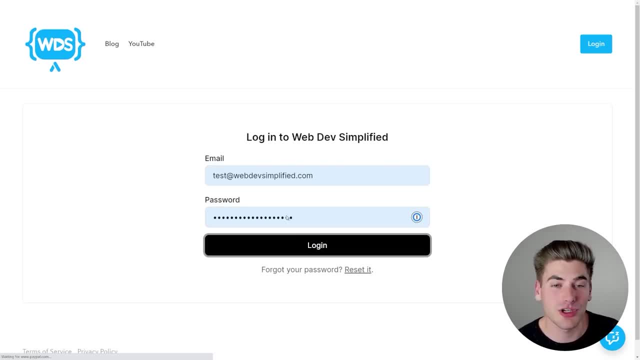 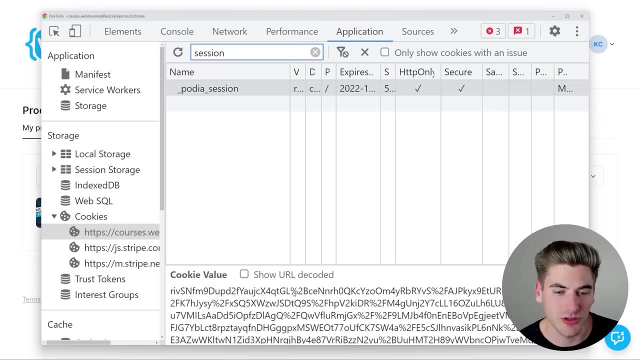 in. So if I just come in here, I log in real quick. what we're going to do is we're actually going to copy that entire cookie. I'm just going to do a quick inspect here. I'm going to go over the application, get that cookie and I just want to make sure I copy it all. So we're just going to. 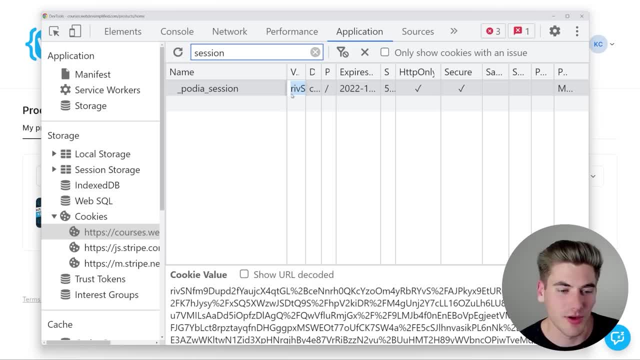 right click. Yeah, I think I can do this. Okay, there we go. That's going to copy the value for that. Then what I'm going to do is I'm just going to open up a brand new tab. We're just going to go. 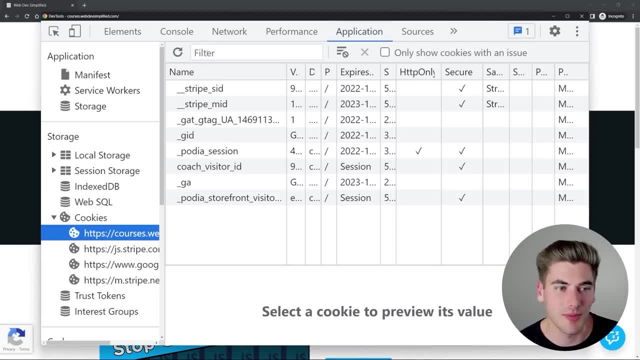 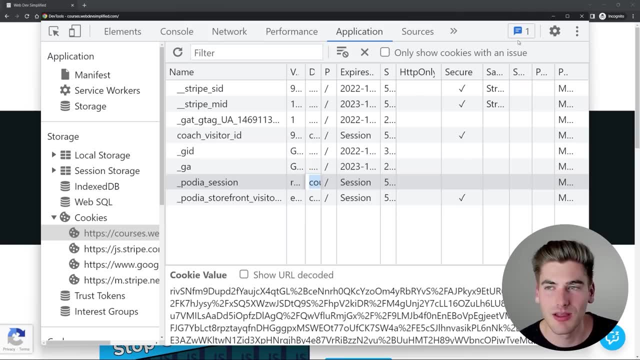 inspect. I'm logged out. Obviously. I'm in a completely new tab. I'm going to come in here, I'm going to create a brand new underscore, podia, underscore session. I'm just going to paste in that value And now, if I just refresh my page, it'll show that I'm actually logged in As you. 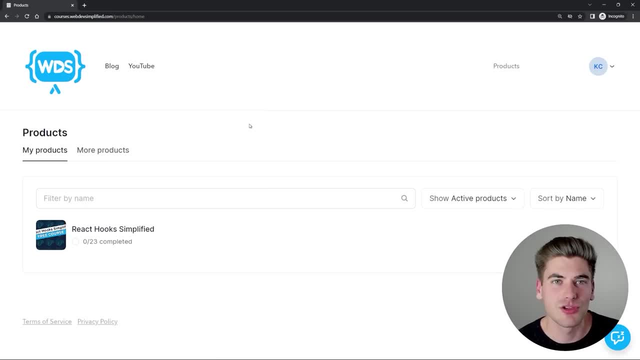 can see, now I'm actually logged in, I can view all the different products that I want to. So it's really important that you make sure you securely store this session ID, because if someone else has access to it, they can be logged in as you without even knowing your username and password. 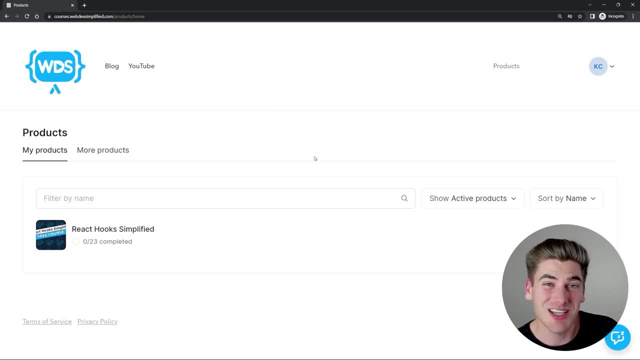 I was able to log in without using my username or password, So this session ID almost acts as like a username password combination that shares and verifies that you are currently who you are, And that's the whole idea behind that. So the next thing I want: 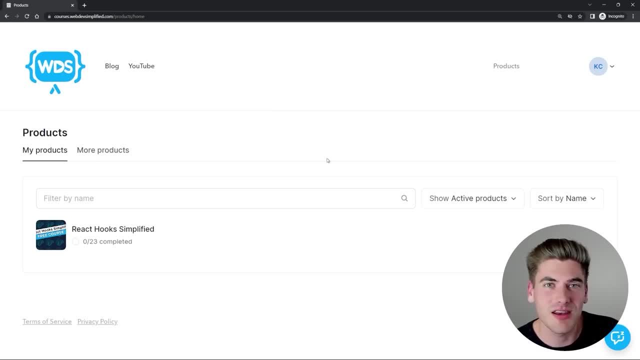 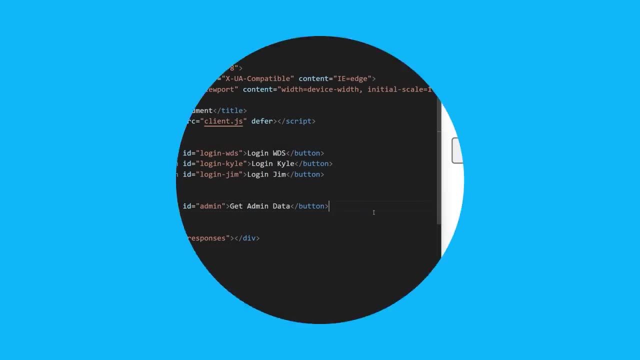 to show you is actually an implementation of how this works on the server side. It is going to be written in Nodejs, but it really doesn't matter. It's going to be super simple code, So the language itself is not at all important. So here I have a really simple application. I have three 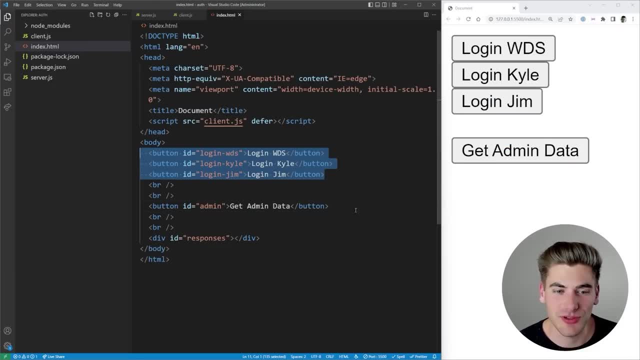 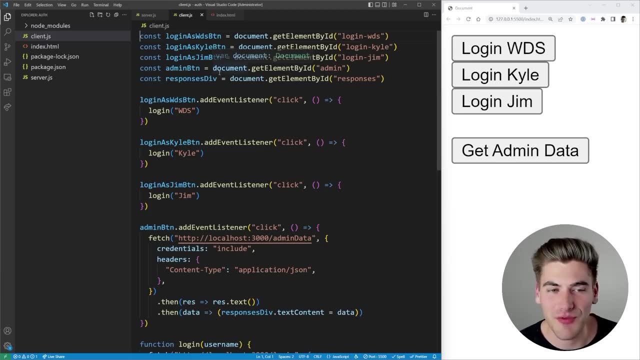 different buttons that are going to do my different logging in of different users. I have a button to try to query some admin data And then I have just a div to show the response of what's happening On my client. everything is really simple When I click those buttons I'm going to 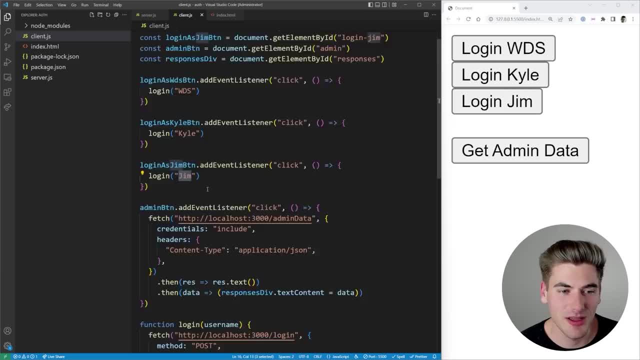 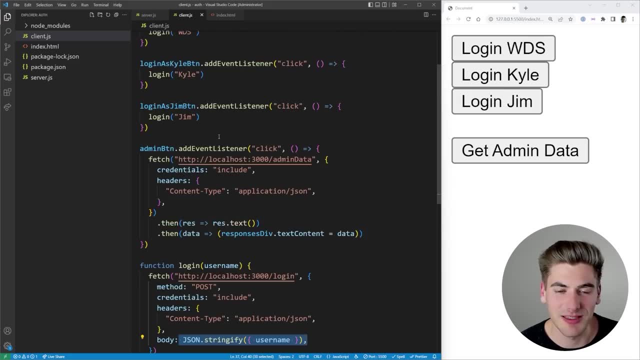 be calling login with the username WDS, Kyle or Jim, And that login function just makes a fetch request to my server, which is just going to pass along our username. Then we have this button to get the admin data. Again, it's going to make a fetch request to my server and it's going to try. 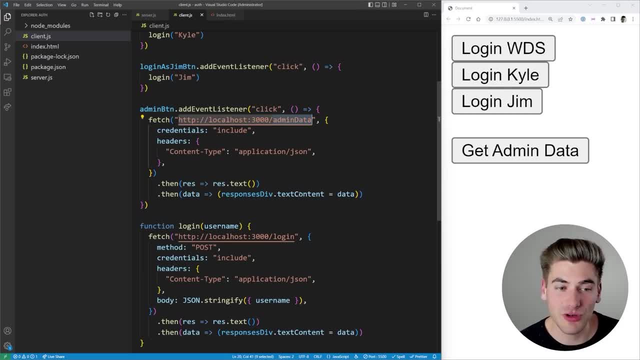 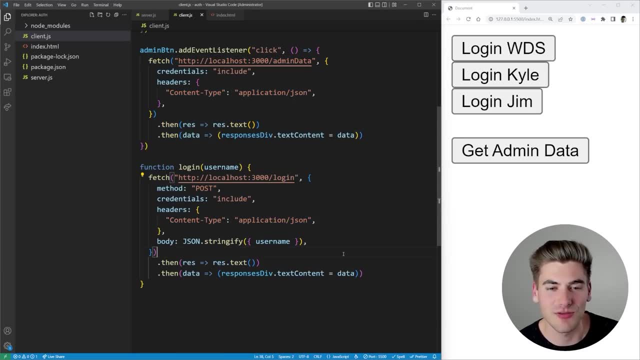 to get the data that is in that admin data route. Now these fetch requests right here. the important thing about these: these are like the requests that are being passed off to the server. So when I try to log in, I'm making a request to the server. that's saying: 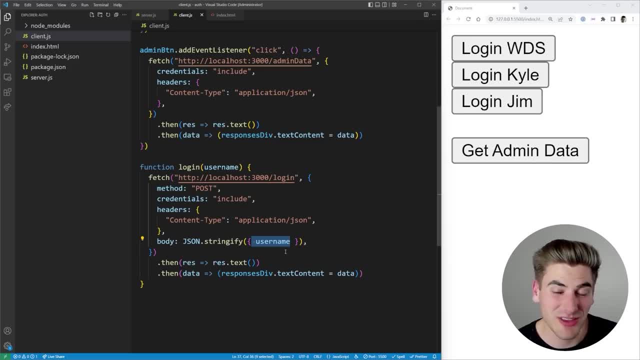 hey, try to log this user in with this username. I don't have any password authentication in this application. It's not important. but if you want to learn how to do password authentication specifically, I have multiple tutorials covering that. I'll link in the cards and description of 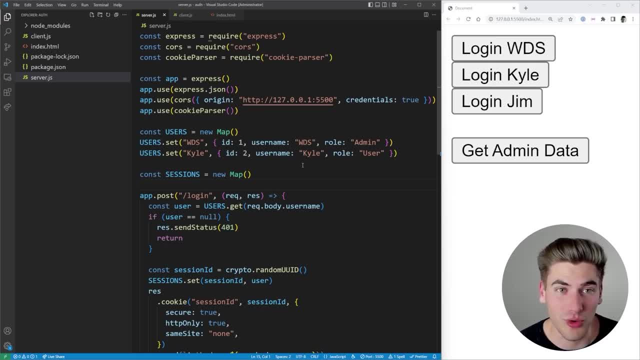 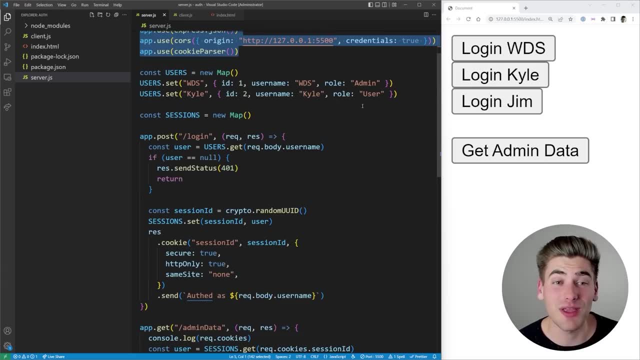 this video. Now, if we jump over to our server, this is where pretty much all of the important code for this project is going. We just have some setup code up here. We're setting up cores to make sure cores works, and just more setup code. Here we have our user database. This map right here is: 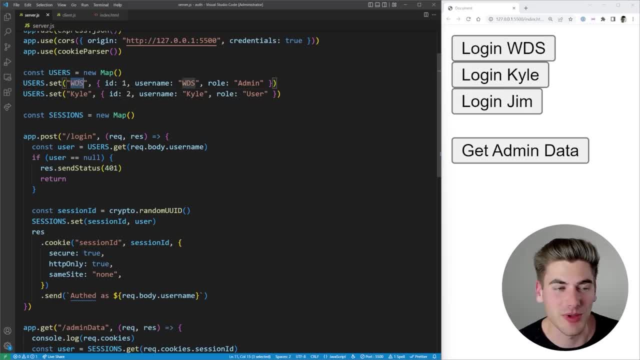 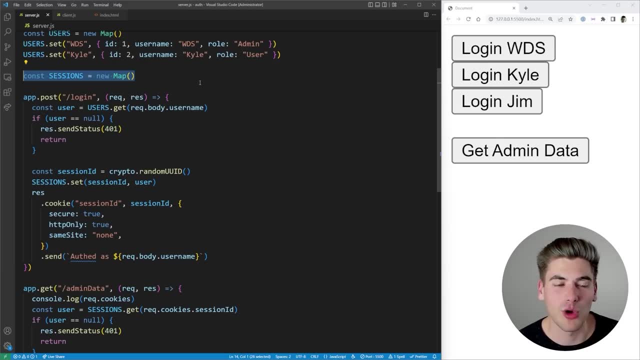 essentially simulating our database of users And we only have two users. We have WDS and we have Kyle. WDS is an admin and Kyle is just a normal user. Then we have a map that stores all of our sessions because we have these unique session IDs, like I showed on my actual website. 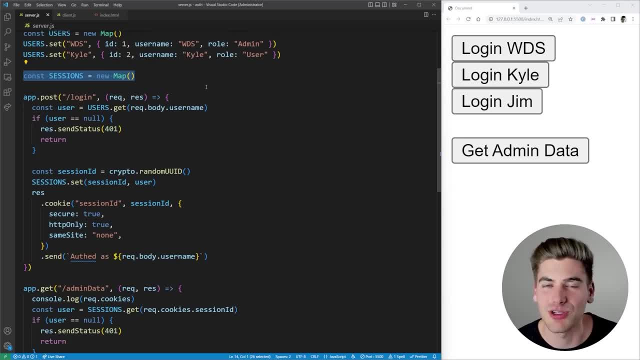 for my courses, And these session IDs are what verify that you're actually logged in and determine which user is corresponding with which session. We need a way to link those two together, which is what this is going to do. So let's look at our login route right here. What we're going to do is 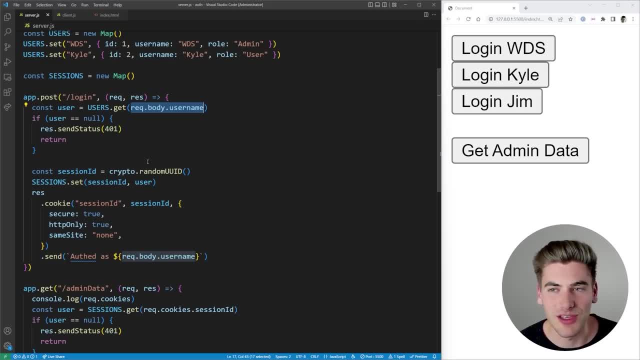 when we log in, we're going to take the username and check to see if we have a user with that username. Now if you did password verification, you would have to check that as well. We're just getting our user. If we don't have a user, we return a 401 status code which says that you. 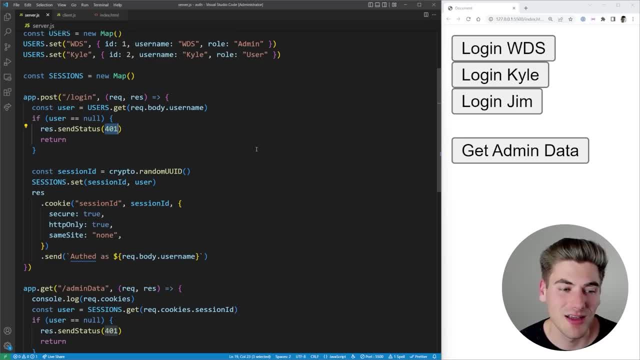 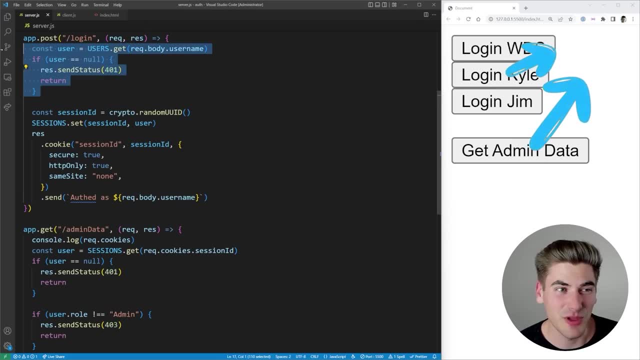 are not authenticated to access this because your data is incorrect. And if you want to learn more about these HTTP status codes, I have a full video on them. I'll link in the cards and description for you. Next, if we are a user, then we're going to create a session for that user. I'm just getting. 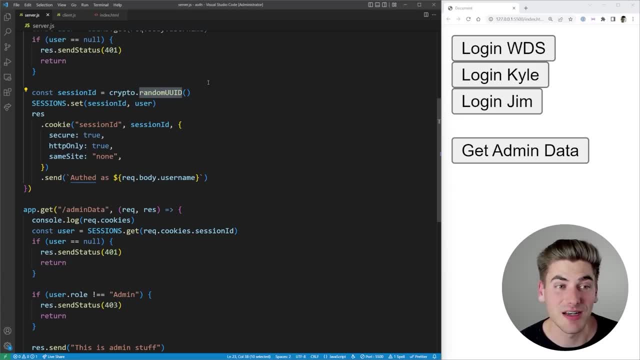 a random UUID, It doesn't really matter- just some type of unique identifier for that user, And what I'm doing is I'm just setting that session for the user And then- this is important part- I'm sending down a cookie and this cookie is secure, HTTP only, And I have same 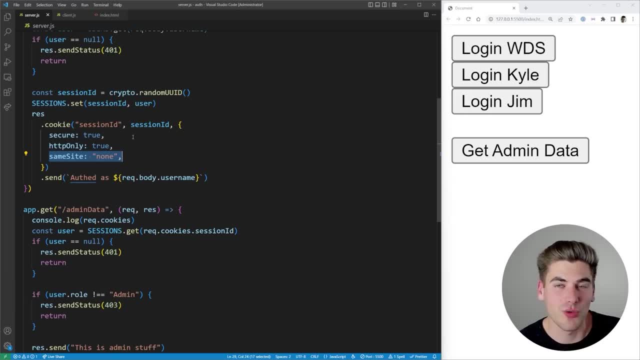 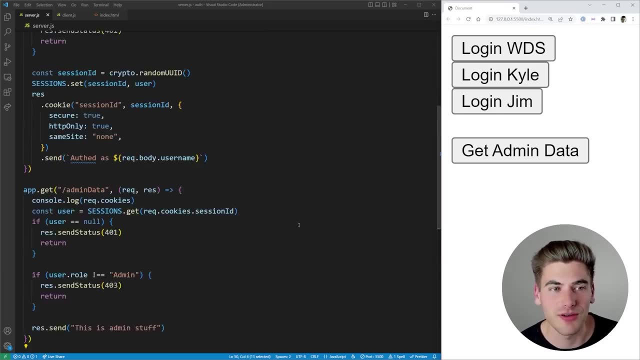 site set to none just because my server and my client are running on different URLs. They're on different ports. I have ones on port 3000, as you can see, and my site up here is running on port 5,500. So this is important: if you're running on a different URL, that you need to set this to. 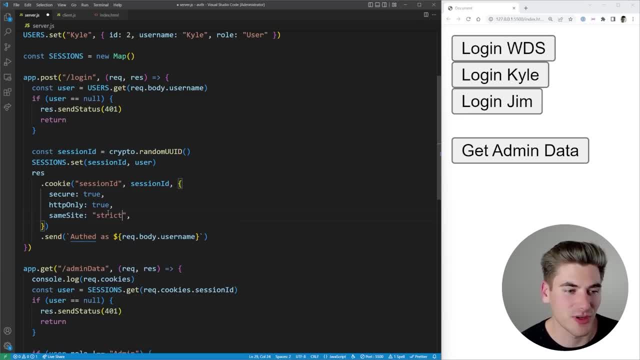 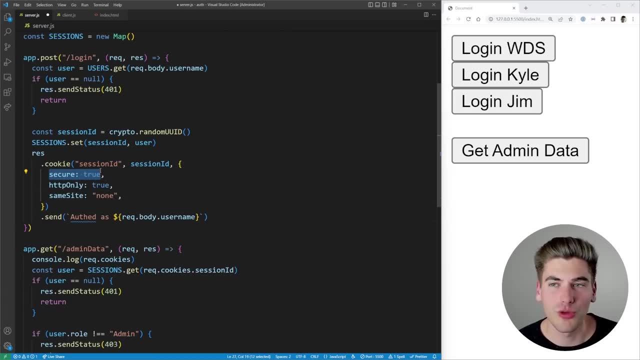 none, Otherwise you can set it to same, or what is it set to? Yeah, strict, And that means it's always going to be only for the same site. So in our case, we need none here. So this is really important. Secure means that it can only be used on HTTPS sites, which is, you know pretty much. 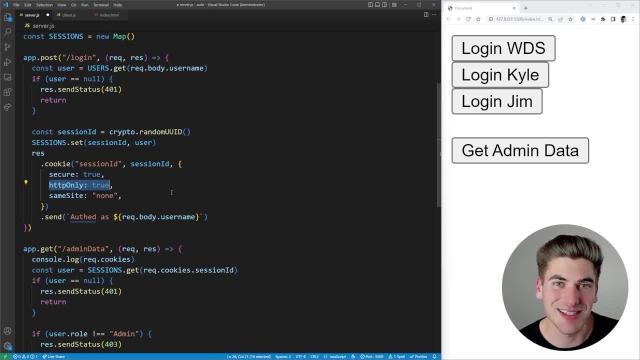 any site should be that way, And HTTP only means you cannot access this via JavaScript. The client cannot access this cookie at all. This is really, really important because it means that you can't actually accidentally leak this data because nobody that has access to JavaScript on your. 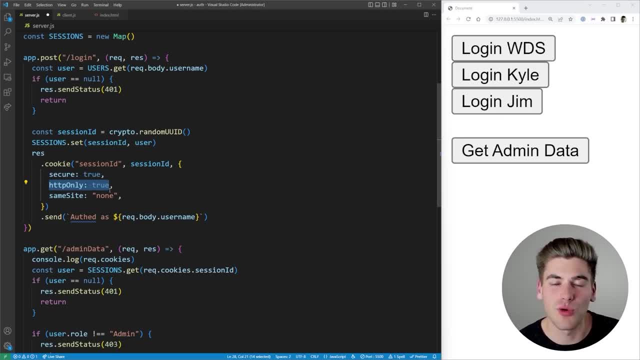 site has access to this. It only gets sent along to the server, So only HTTP requests have access to this session ID. This is really important to understand and why you should always or these types of sessions in a cookie and not in some like local storage or session storage. 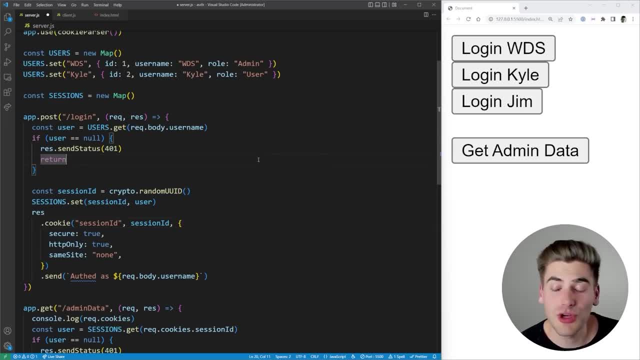 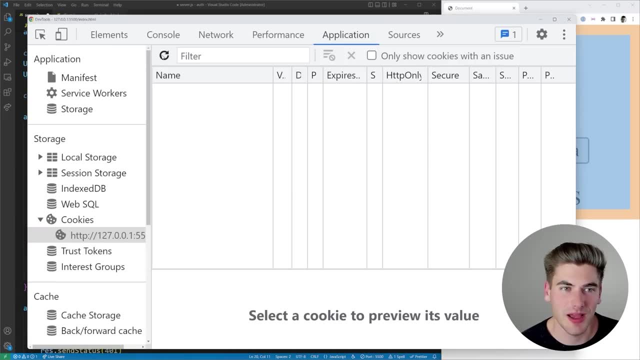 Then I'm just sending down the text that says you're off as that user. So to show this working, let's just refresh our page here and click in login- WDS. You can see it says off as WDS. And if I inspect, go over to my application here, which do this real quick. again, refresh with the. 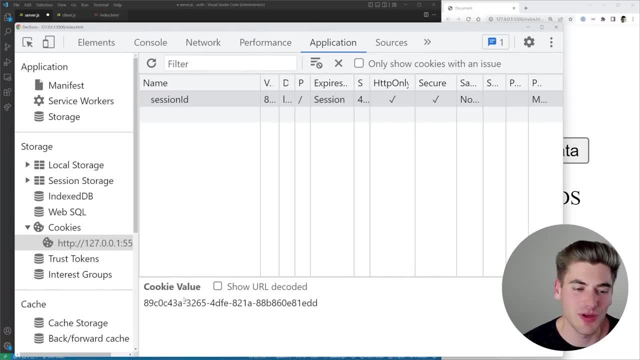 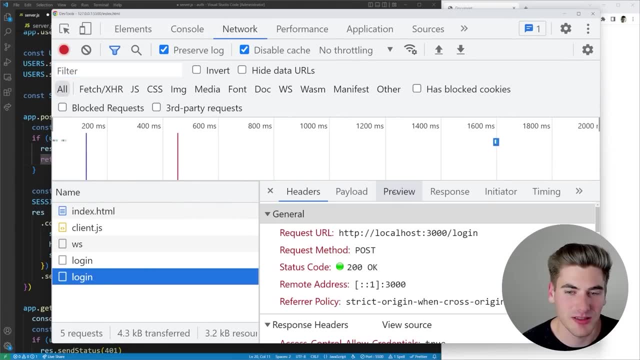 login button. There we go, Go over to application tab. You can see we have a session ID with this value And this value is just a random UUID that's generated on the server and our network. You can see we actually have that login request. 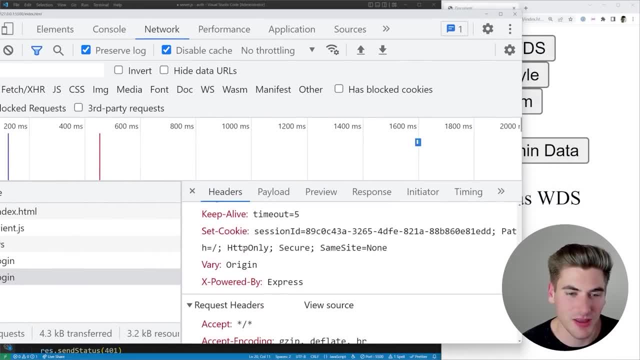 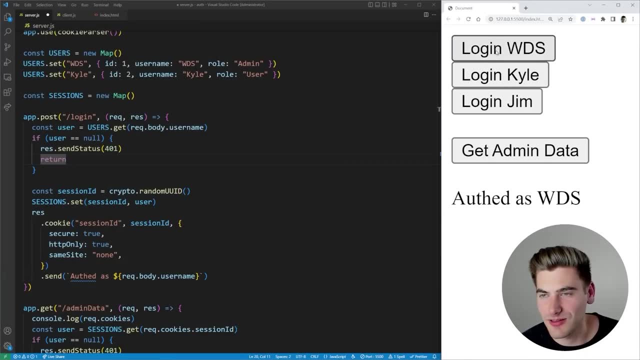 And if we look at the headers, you can see here that we have a cookie being set is saying: Hey, set this cookie, which is the session ID. So it's being passed down from the server, which is great. So we can do that as WDS, We can do it as Kyle, but if we click on login Jim, there is no Jim. 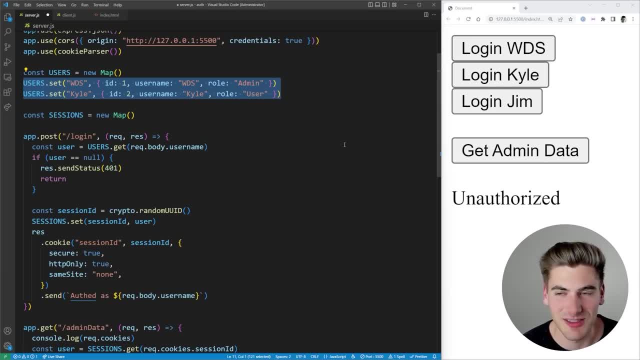 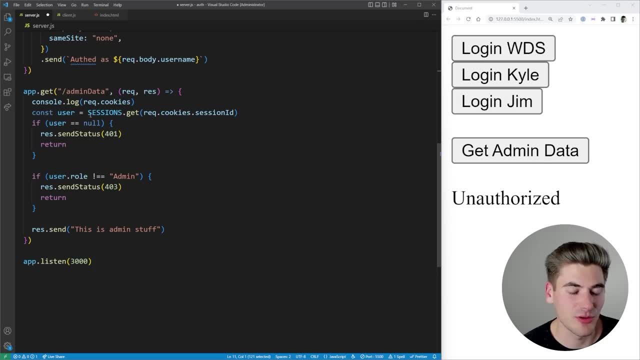 user. So we're getting that unauthorized error being sent to us saying that Jim does not exist as a user. Now the next thing that we have in here is this: get admin data And to do this, what we're doing is we're passing or we're checking our session. sorry for the cookie. 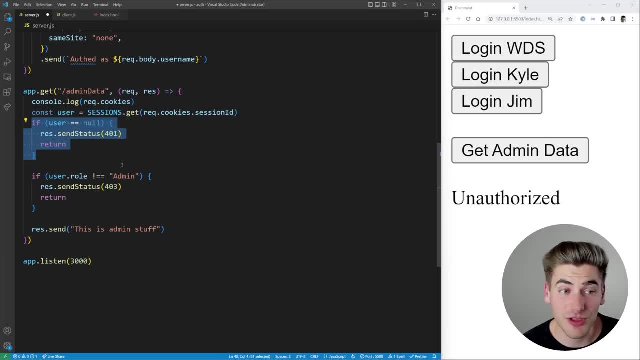 That is our session ID, And then, if we don't have a user, we're going to have to go to our session ID. And then, if we don't have a user, that means that we either passed up no session at all or the session that we passed up doesn't actually match up with any of our sessions. In that case, 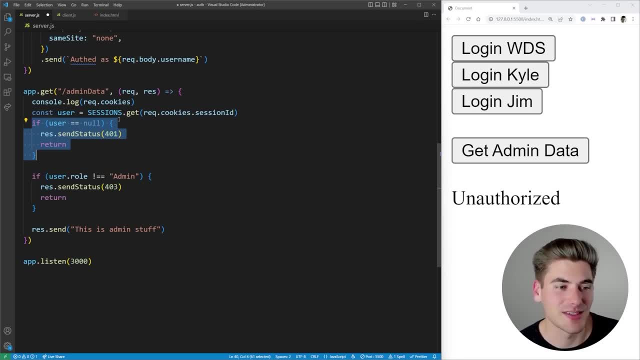 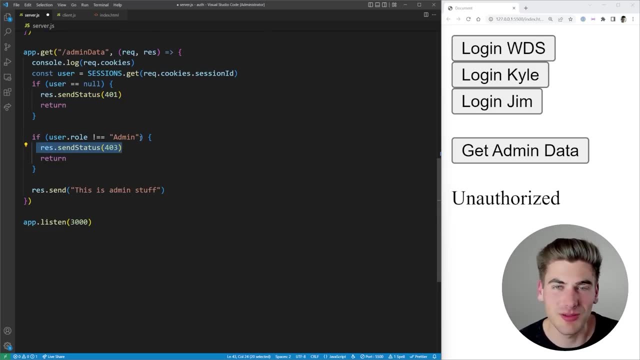 throw down an error that says you're not authenticated because you don't have a session. If you do have a session and you want to check your role to make sure that you're an admin, if you're not an admin, we're going to throw down a 403, which means you're not authorized to access. 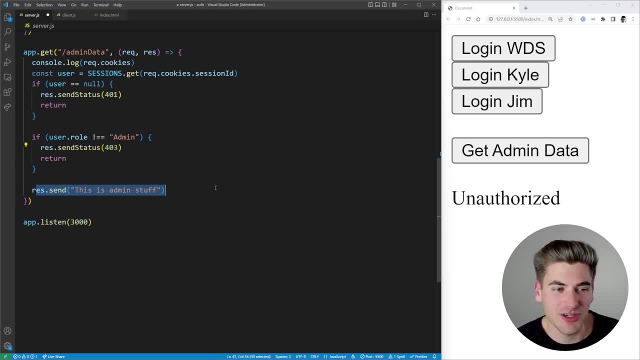 that information because you don't have the correct permission. Otherwise, we're just going to send down all of our fancy admin stuff, which is just a simple string. So if we test how this works, I just refer back to that And then we're just going to send down all of our fancy admin. 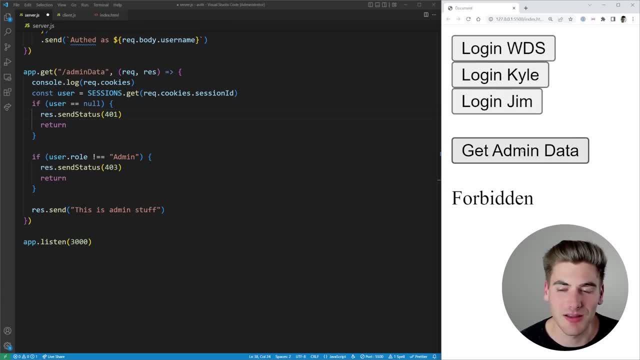 stuff, which is just a simple string. So if we test how this works, I just refer back to the page Let me log in as Kyle and I'm going to click get admin data. You can see it says forbidden, because while I'm logged in as Kyle, Kyle is not an admin, He's just a normal user. 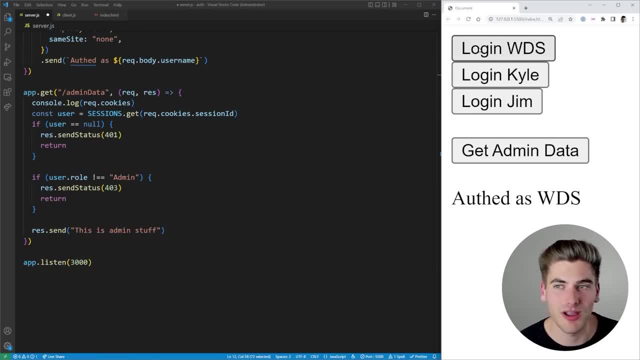 So he does not have access to the admin stuff. I just do a refresh, log in as WDS and click get admin data. You can see I get it just fine because I'm authorized to get that information. Now the one important caveat to make sure all of this is working just fine is, if you need to, 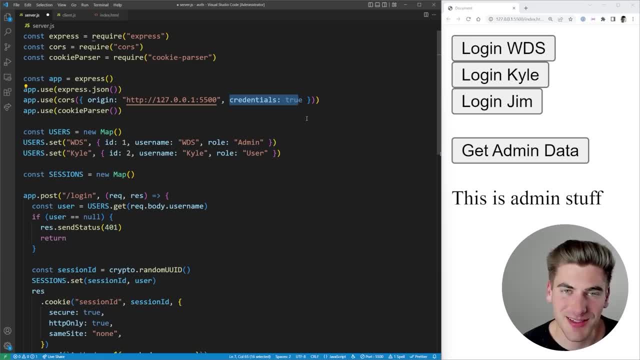 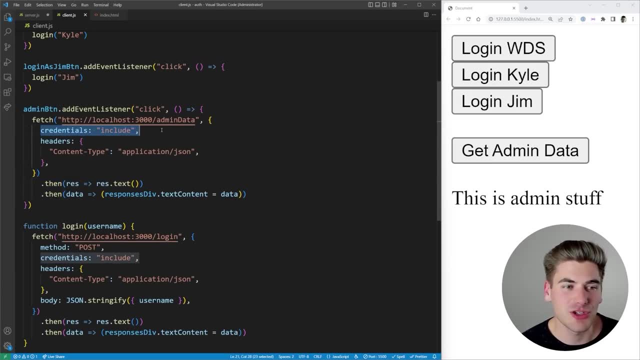 use cores. when you set it up, make sure you allow credentials to be passed. That essentially stands for cookies. You're allowing your cookies through and on the client. whenever you make a fetch request or Axios or whatever you're doing, you need to make sure that you include the 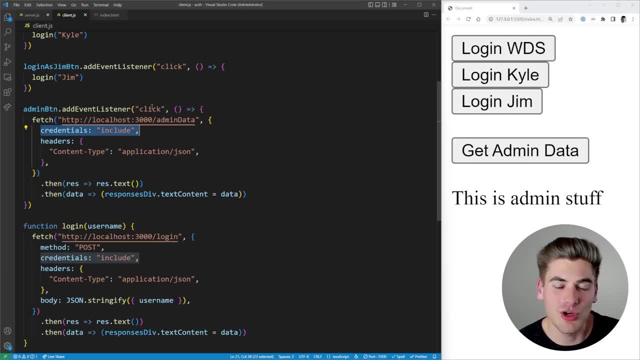 credentials by passing this line right here. That's going to make sure that the cookies get passed along with all of your different requests. Otherwise they don't get passed along by default. If you remove this line, nothing at all is going to work. Now also to recap exactly: 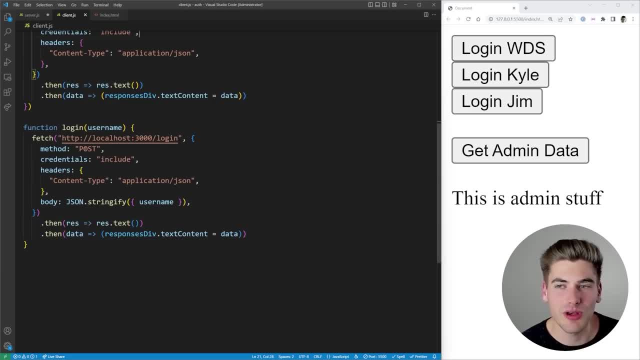 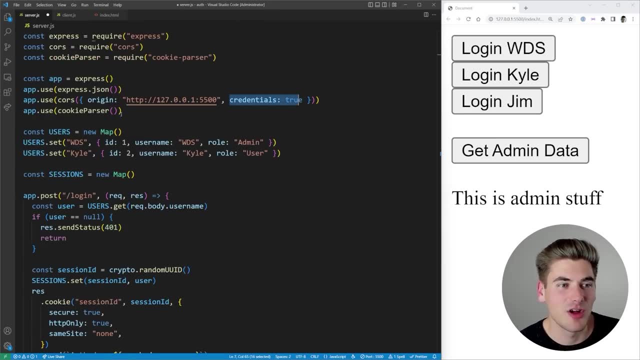 the process of how this works. what happens at the very beginning is we're going to be trying to send a request from the client to the server saying: log me in with this username and password. In our case, it's just a username On the server. we're getting that information and what we're 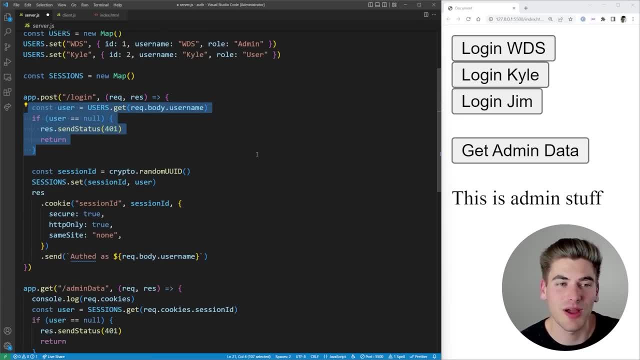 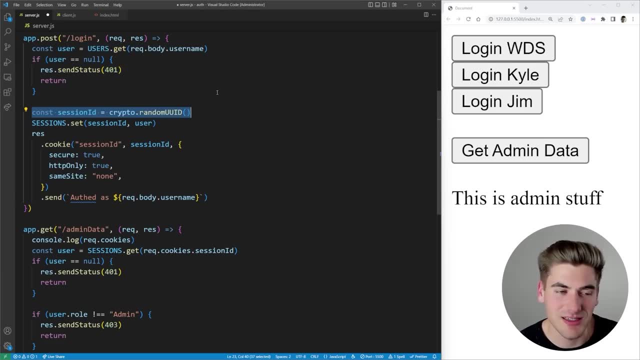 doing is we're checking to see if this user's login credentials are correct. If they are not, we send down an error. If they are correct, we create a new session ID for that user. However you want to create that session ID, it doesn't matter, But the important thing is we save that. 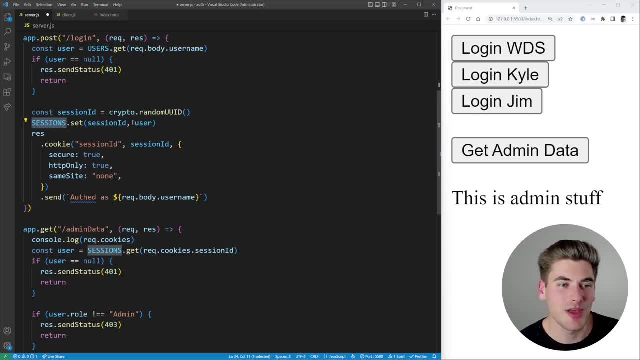 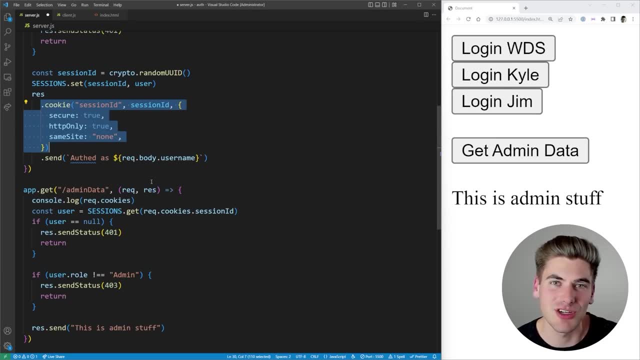 session ID somewhere- usually somewhere like Redis, for example- and we make sure we tie the user to that session ID- That's the really important part here- And then we send down a cookie that's saying: hey, this is your session ID for you to use throughout all of your different. 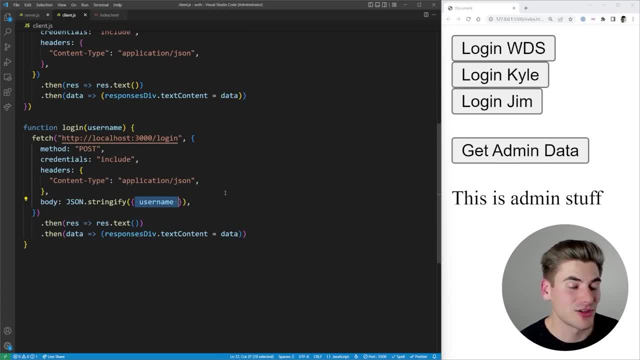 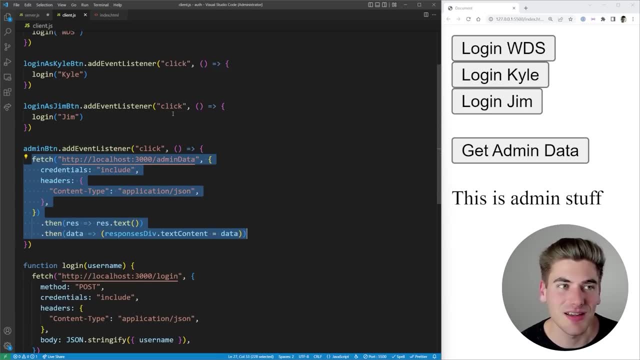 you know uses of this application. Then, back on the client, you know stuff is happening and now the user wants to get some data- protected data. Well, we're going to send along a new request that says you want to get that data. And on the server what we're going. 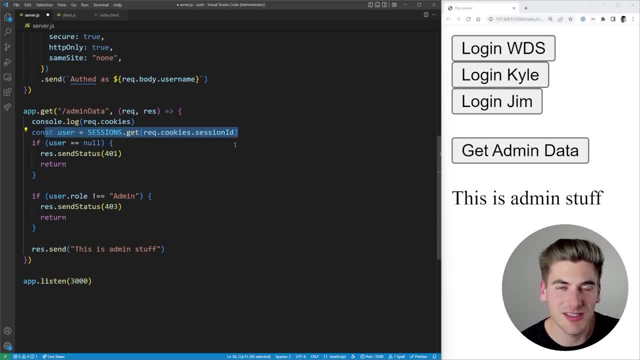 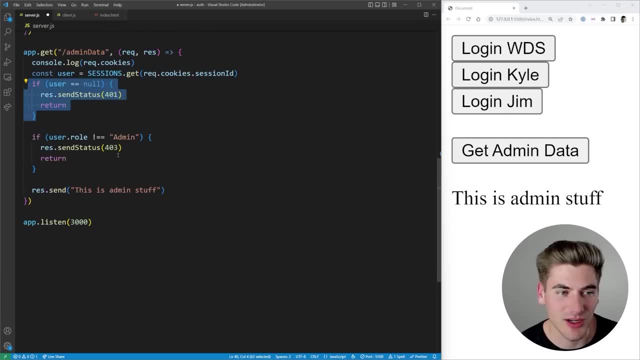 to do is we're going to get the user from that session, because we stored the session and the user together using this code right here. So we're going to get the user from our session. If there is no user, obviously no one's logged in If the user doesn't have the correct permissions. 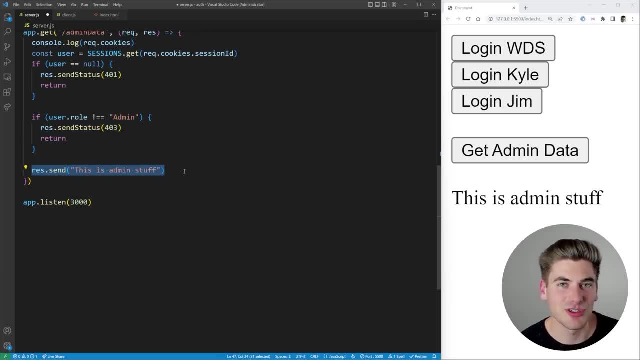 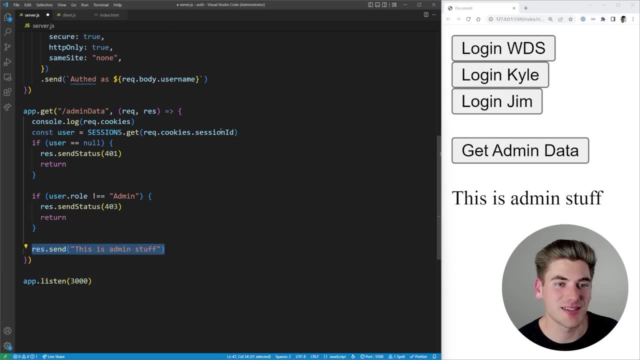 we throw back any necessary errors And then, based on the user's permission, we show them the stuff that they have access to or allow them to perform some action that they're attempting to perform. The really important thing to understand here is that this session ID essentially 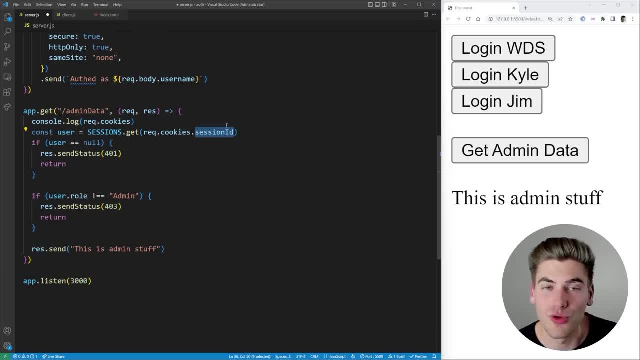 acts as like your login credentials. This is like you saying who you are. That's what the session ID is doing, So it's really important that we make sure we keep that secure and that we don't leak that anywhere on the web, because otherwise people can access and use your account using that session. 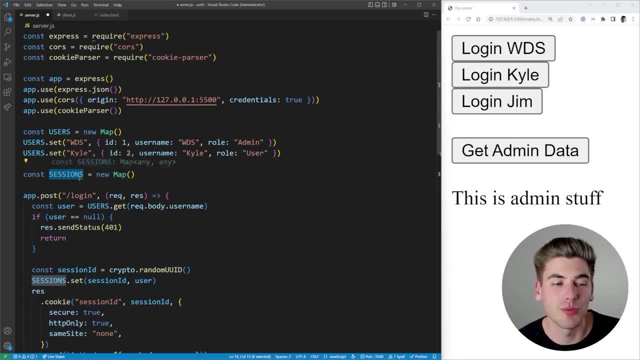 ID. That's why, generally, it's a good idea to make sure you periodically remove current sessions from your session map. So if a user has been inactive for a certain period of time, we've removed that session. Think about if you've ever logged into a bank account and left it open on your screen. 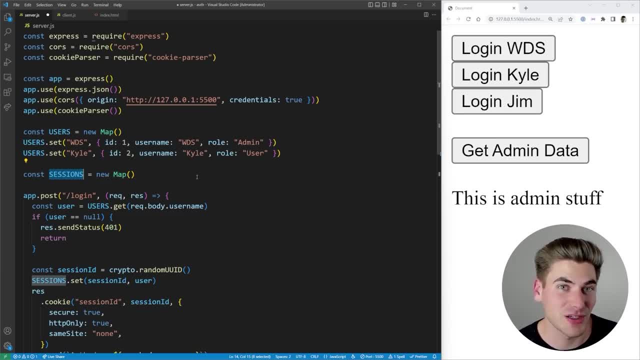 for a while. it'll usually pop up a message that says: Hey, if you're inactive for five more minutes, we're going to, you know, log you out automatically. The way they log you out is by removing the session from the server. That's all that they do. The final important thing to: 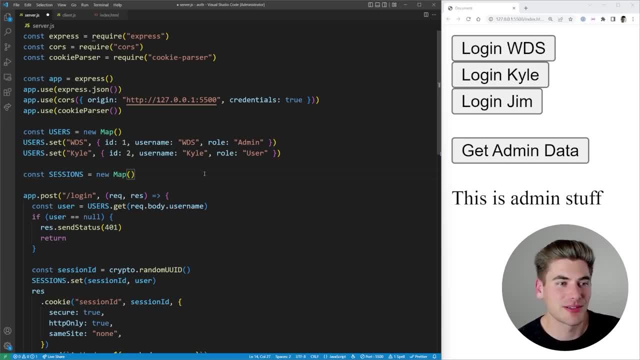 understand about authentication is most of all of the complex stuff around. dealing with sessions and cookies is almost always going to be handled by some type of library. For example, express has their very own express session library that handles all that for you. Nextjs has like their. 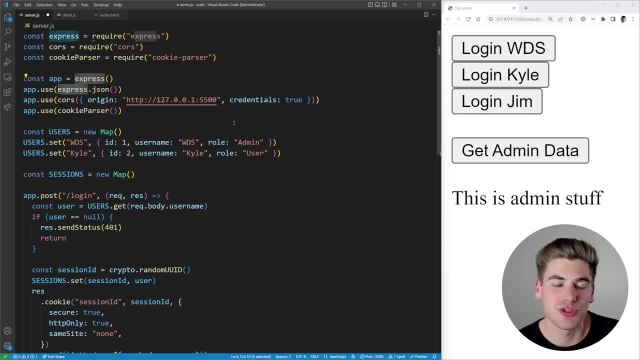 own next off that you can use pretty much any major framework or tool out. there is going to have some library that makes dealing with this so much easier, So I'd recommend just using that. but it's also nice to understand exactly how it works behind the scenes So you can easily troubleshoot. 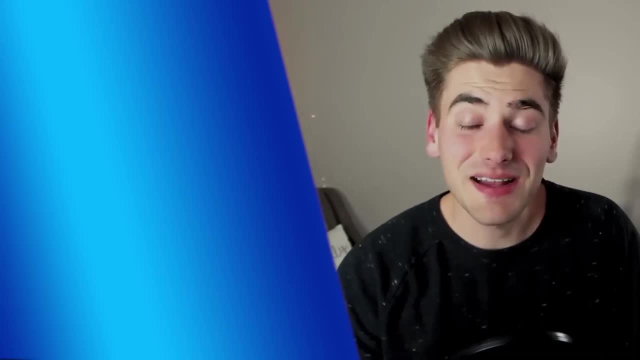 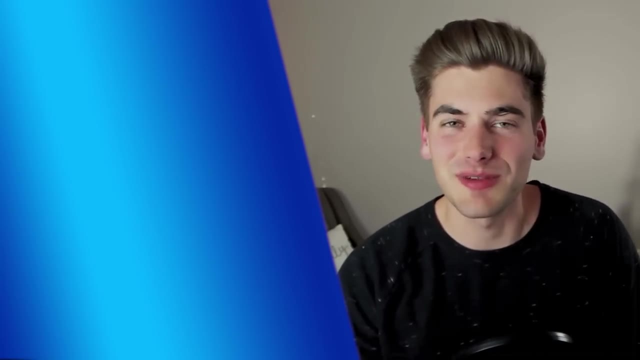 things or add on new features if you need them. And that's all there is to understanding it off. If you want to go even deeper into implementing specific off things like JWTs or username and passwords, I'm going to have videos on those linked right over here. And with that said, thank you very much for watching and have a good day.